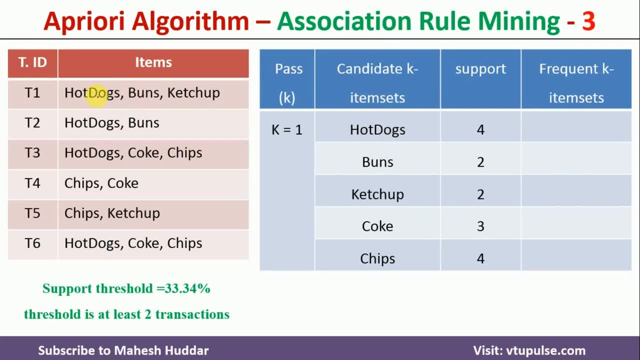 these items were purchased. If you see here, hot dogs is purchased 123 and then four times. That is what I have written here. Similarly, buns- buns is purchased two times, So I have written it here. Similarly, we have to count the number of times each and every product was. 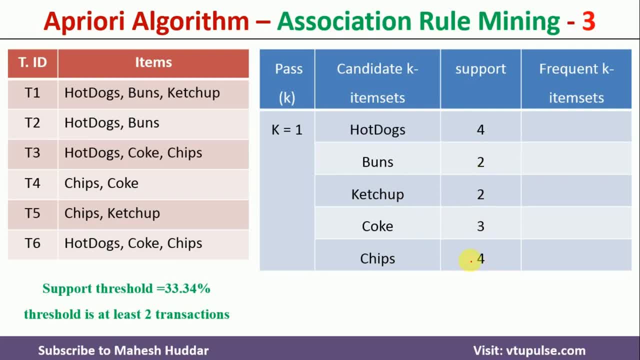 purchased in this case. Now, if you see this particular support value, every item will satisfy the minimum support because minimum it has to be purchased two times in this case. So all of these will satisfy this particular requirement. The meaning is: all are. you can say that the frequent 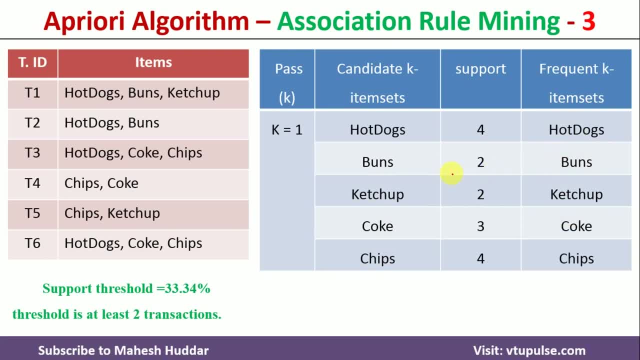 one item sets in this case. Now, what we need to do is we need to write the two item sets first. that is case equal to two in that case, To write that we will start with hot dogs, hot dogs, buns, ketchup. 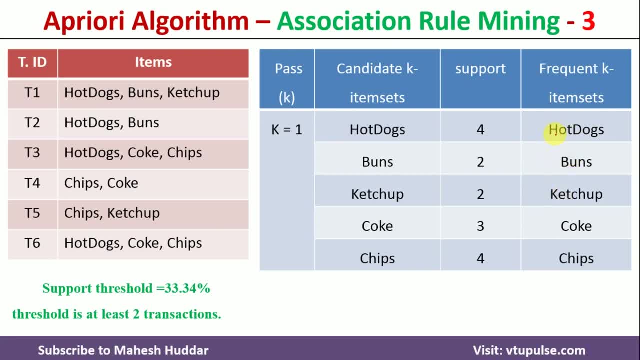 that's the first one. Hot dogs and ketchup is the second one, hot dogs Coke is the third one, hot dogs chips is the third, fourth one, and then we will start with the buns: Buns ketchup, buns Coke, buns chips is the next three possibilities. 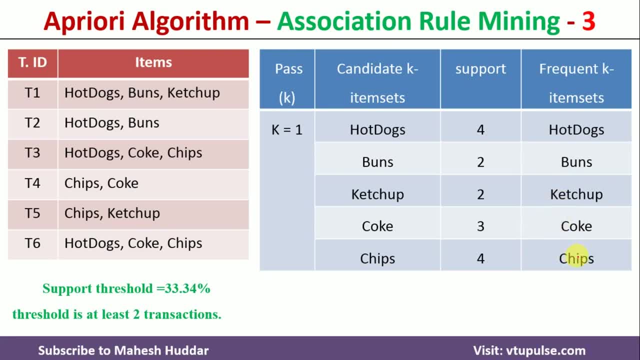 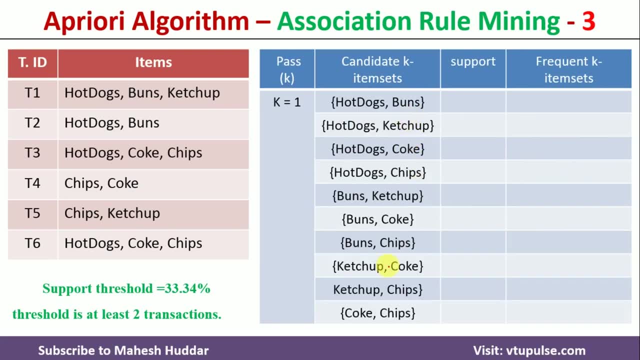 Ketchup, Coke, Ketchup chips is another two possibilities, and the last possibility is coke chips will get 10 possibilities. so that is what i have listed here. in this case the k is equivalent to to here. now we have to find out the support value, that is, how many number of times this? 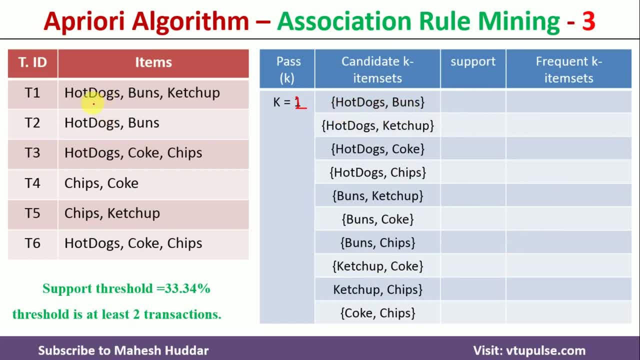 hot dogs and buns is purchased. if you see, here, hot dogs and buns is purchased one time, here this is the second time, so it is purchased two times. similarly, we have to find out the hot dogs and ketchup. this is hot dogs and ketchup. this is the first time. we don't have any other possibilities. 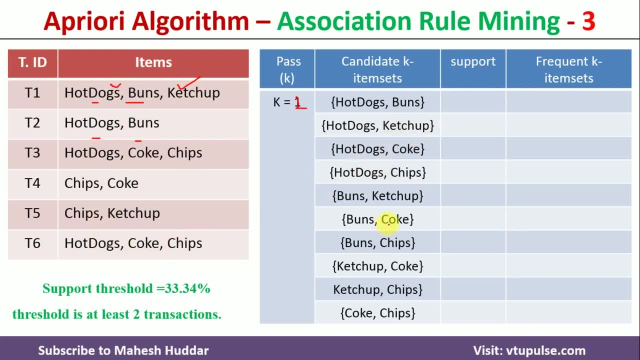 the meaning is: it has been purchased one time, the. similarly, we have to count the support value for all these particular possibilities. you can see here, the first one was purchased two times. second possibility is one time, and so on. we have listed all these things. now, out of all these particular 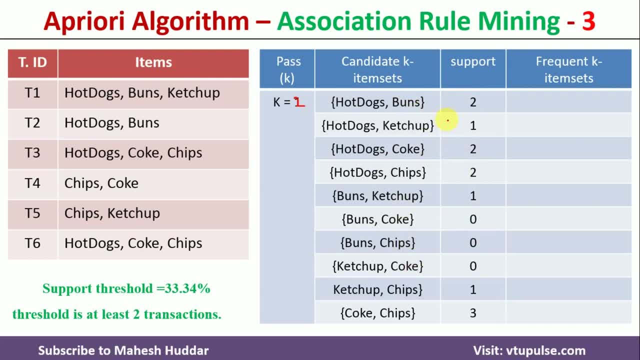 possibilities? uh, the one which will satisfy the minimum support. that is two we have to consider here. this is the first one, second one, third one and then the fourth one here. so these are the frequent two item sets in this case. so that is what we need to write. so it is two here now. uh, these are the frequent two item sets. 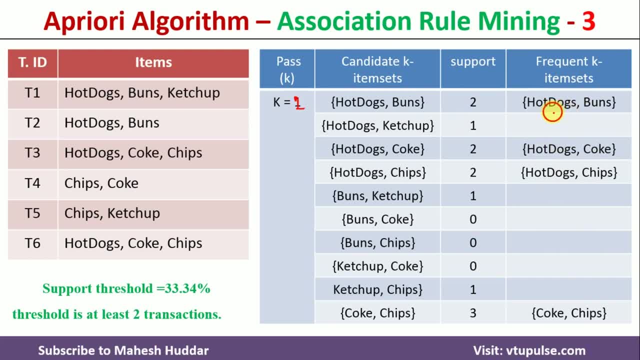 uh, in this frequent two item sets, if you see here. uh, this is the first unique item: hot dogs, buns, coke chips. these are the four possibilities. now, by considering these four, we have to write the three item sets. so these are the four possibilities first. so how to write is: 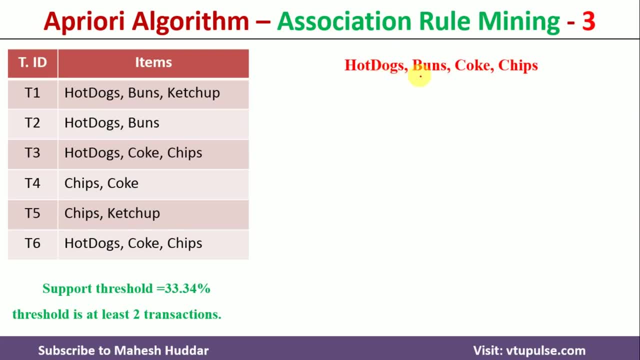 we have to start with again. hot dogs- hot dogs- buns coke- that's the first possibility. hot dogs- buns chips is the second possibility. hot dogs- coke chips is the third possibility. buns coke and chips is the fourth possibility here. so these are the four possible cases. 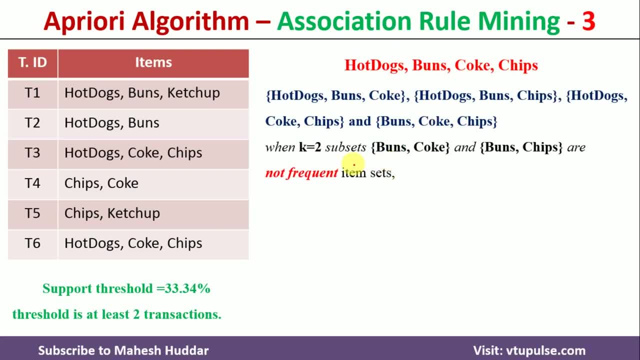 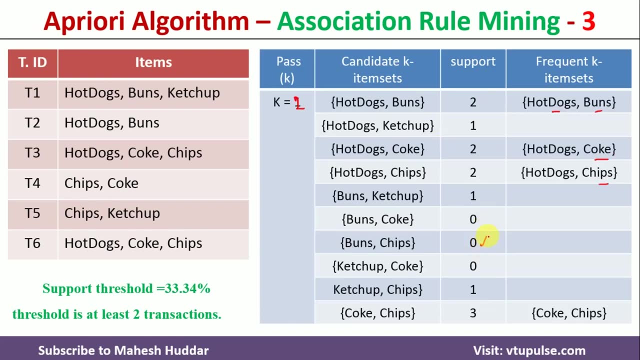 but if we consider, you should not consider all four possibilities, because when k is equivalent to 2 here the buns and coke is not a frequent to item set. similarly, buns and chips is not a frequent to item sets. if you go back and see here buns and chips, we have zero and 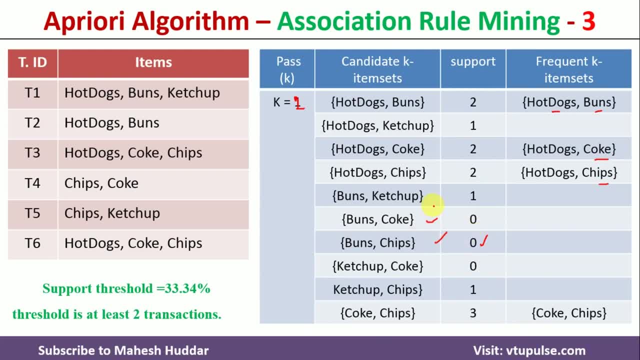 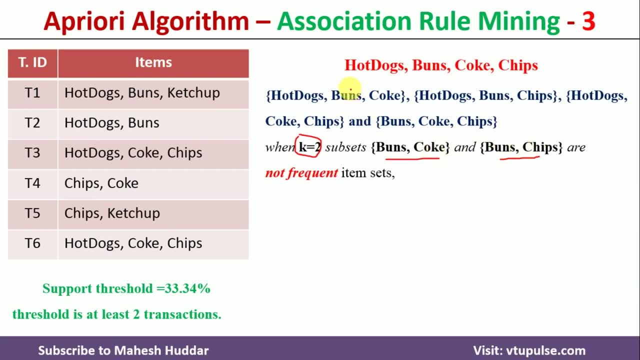 buns and coke is equivalent to zero here, so these two are not frequent to item sets here. so what we do here is: wherever these two are appearing, we will remove those things. so bun and coke is appearing, so we should not consider this one. bun and chip is coming, we should not consider this one and then 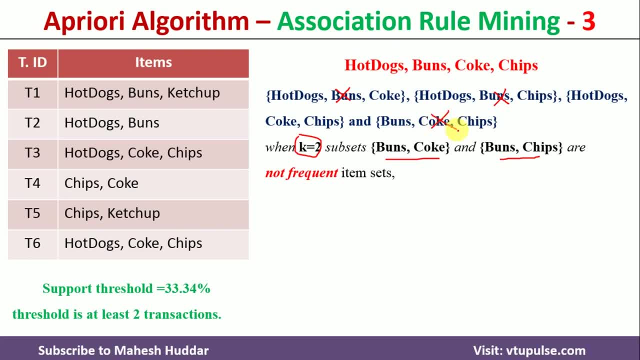 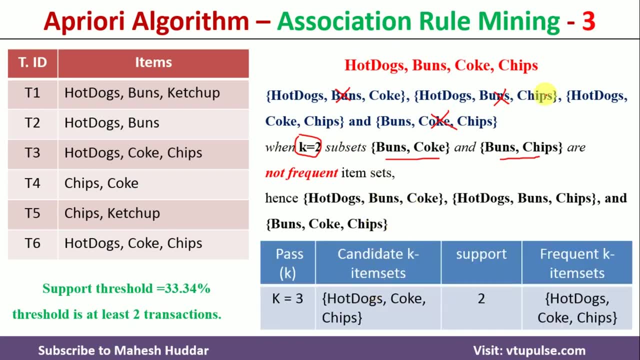 bun and coke, as well as bun and chip, is appearing here. i should not consider this one. so there is only one uh three item set we have. uh, we should not consider all three. we have only one, that is, hot dogs, coke and chips. so this is the only item set that we have. we should not consider all three. 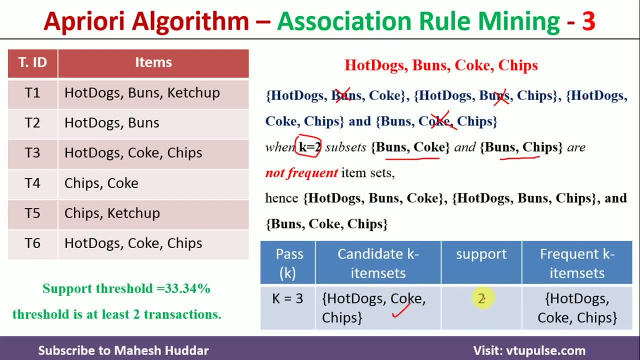 only- uh, frequent three item set in this case, where the support is equivalent to two, because we need to count it here: hot dogs, coke chips. this is the first time, hot dog, coke chips. this is the second time, so it is appearing two times in this case. so the minimum support has been satisfied here, so 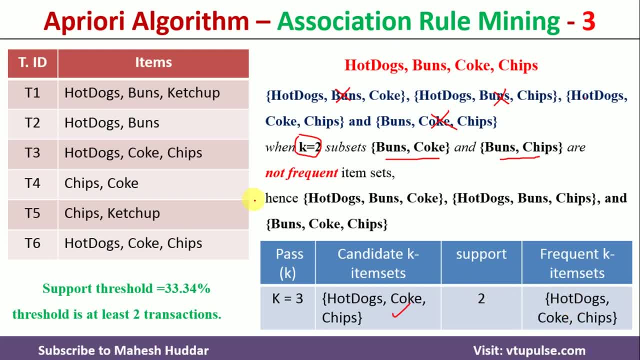 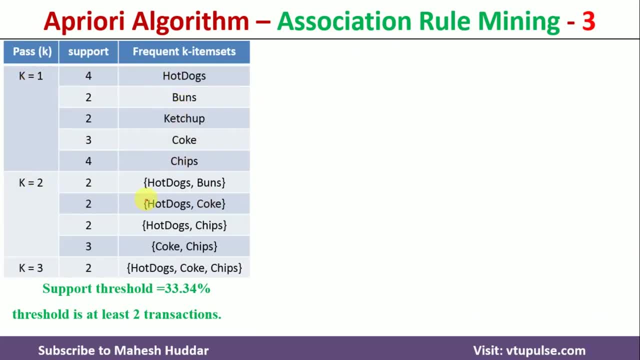 this is the frequent three item set here. once you find out this particular frequent item set- uh, this is what we calculated when k is equivalent to one. these are the item sets when k is equivalent to three. this is the item set here. now, what we need to do here is, uh, we have to find out the 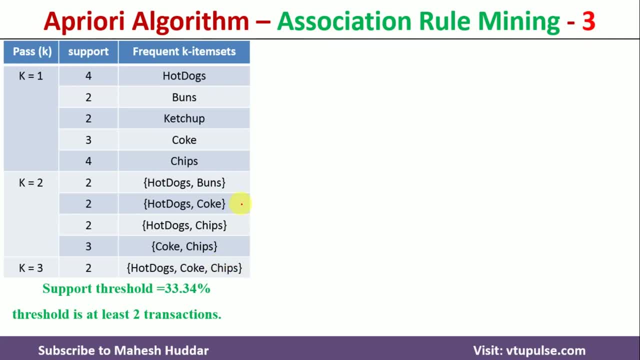 association rules, and then we need to find out the strong association rules based on the confidence value. so i will start with this one. that is the first frequent item set, because i cannot write any rule with respect to one item set, so i should start with the two item sets here. the first one: 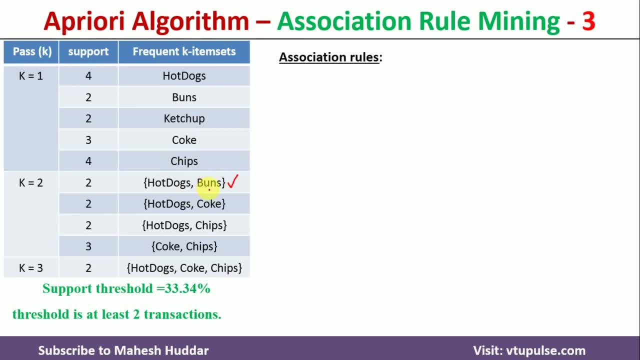 is hot dogs and buns. here. hot dogs and buns can generate the two possibilities: hot dogs, bun, that is the first one, buns and hot dogs. so the first one is hot dogs and buns and the second one is hot. these are the two possibilities. so when you consider this one- hot dogs, buns- here first we 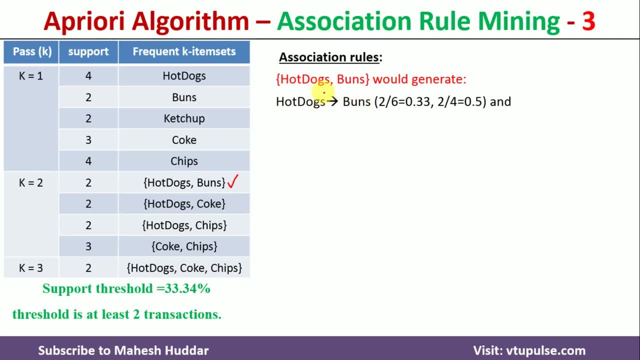 need to calculate the support value of this particular thing. support is nothing but how many times both are purchased divided by by number of transactions here. so if you see, here hot dogs and buns is purchased two times and the total number of transactions are six. so the support 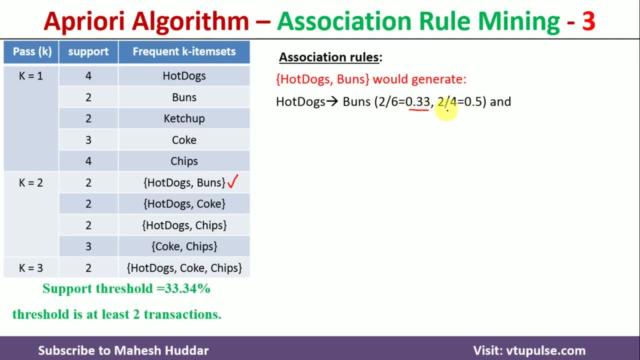 is equivalent to 0.33 in this case. now, coming back to the second one, this is the confidence. the confidence is nothing but the number of times both are purchased divided by the number of times hot dogs is purchased here, so the number of time both are. 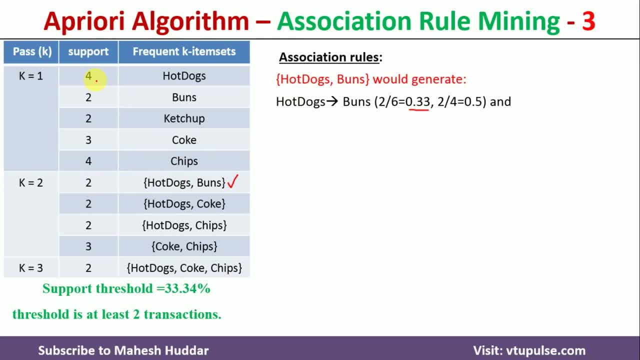 purchased is two divided by the number of times hot dogs is purchased is four here. so two by four, which is equivalent to 0.5, which is less than the confidence. that is confidence is equivalent to the 60 percent in this case. so it is less than the confidence, so we uh will not consider this. 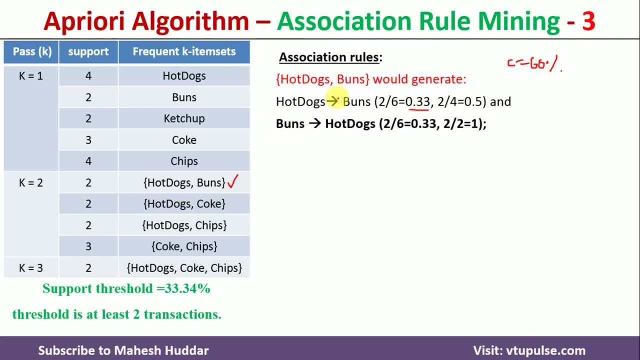 as a strong association rule here. when you consider the other possibility, that is, buns and hot dogs, again the support remains same because the number of times both were purchased is two out of six and the number of times both were purchased is two divided by the number of times brunch is purchased. that is two here. 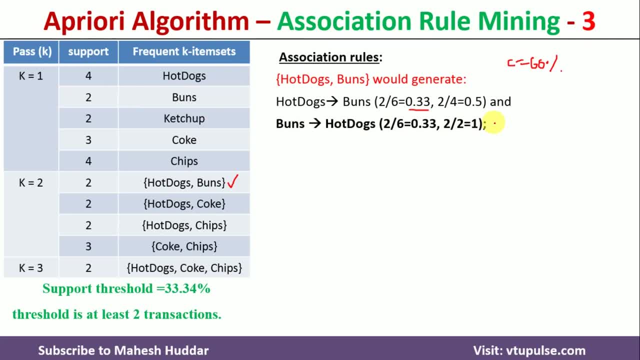 so two by two is equivalent to one. that is hundred percent. so this is a strong rule in this case. this is the first strong rule. consider the second, uh frequent item said, that is hot dogs and coke. it has again two possibilities: hot dogs and coke, or coke and hot dogs. 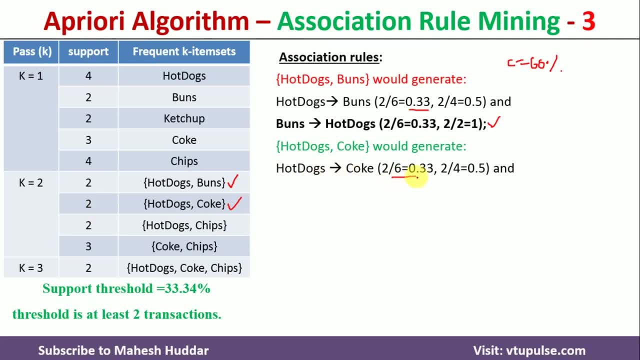 so both are purchased two times out of six. that is the minimum support here. and then confidence is: both are purchased two times and the number of times this hot dogs is purchased is four here. so it will be 0.5 in this case. again, it is less than 60 percent, so we don't consider this as a 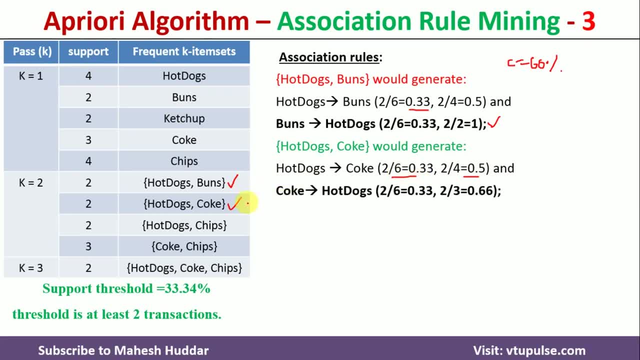 strong association rule. now considering the second one, that is, coke hot dogs. coke hot dogs again. both are purchased two times out of six. and this confidence, that is, both are purchased two times the number of time coke is purchased is, i think it is three times, so two by three that. 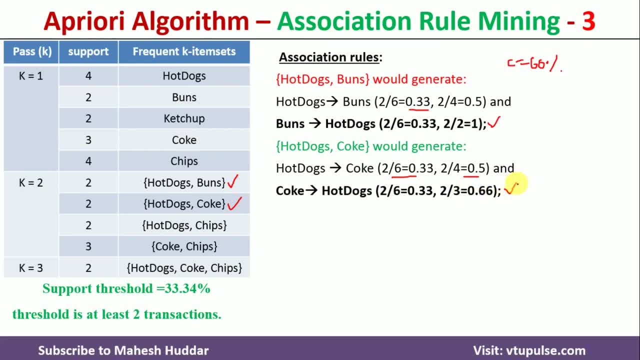 is 66 percent, so it is satisfy the minimum confidence. hence it is a- you can say that- strong association rule. now, coming back to the next one, that is, hot dogs and chips, the two possibilities are: hot dogs, chips, chips, hot dogs, so both of them are purchased two times again out. 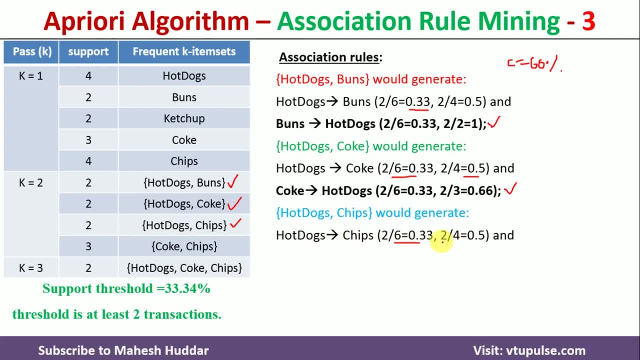 of six. so that is a minimum support. both of them are purchased two times. divided by the number of times hot dogs is purchased, that is four here, so it is 50 percent. again, it is less than 60 percent here. coming back to the second one, chips, hot dogs. both are purchased two times out of six. that is a 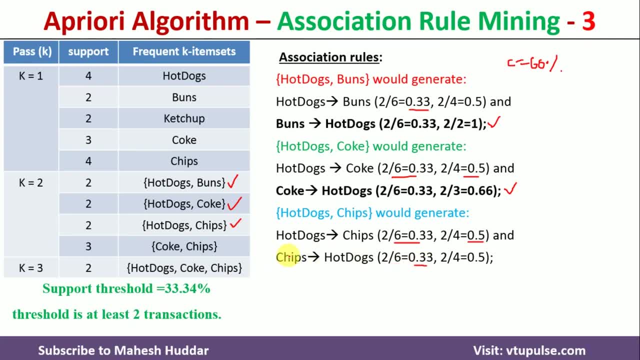 support. both are purchased two times divided by the number of times chips is purchased is four here. two by four, that is 0.5 in this case. again, it is not a strong rule. in this case, coming back to the last one, that is, coke chips, we have two possibilities. coke chips is the the strong rule. 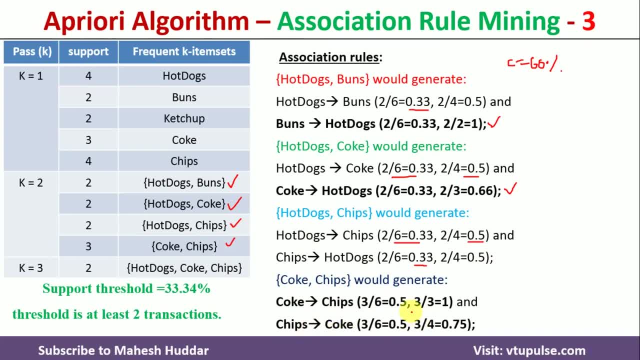 similarly, chips coke is also a strong rule in this case. so this is a strong rule in this case. so this is a strong rule in this case. so, if you see, here we got four strong association rules with respect to two, two frequent item sets. now coming back to the next one, that is, there is 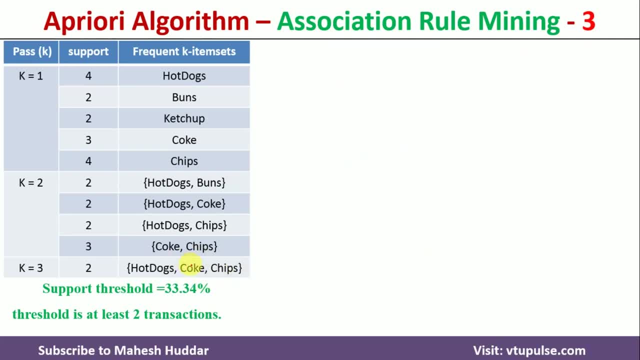 one three frequent items that we have. so we have to write all possible cases. so the first possible case in this case is hot dogs, right side. the remaining two that is coke chips. so the number of times all three were purchased is two divided by the number of transactions. that is support here. 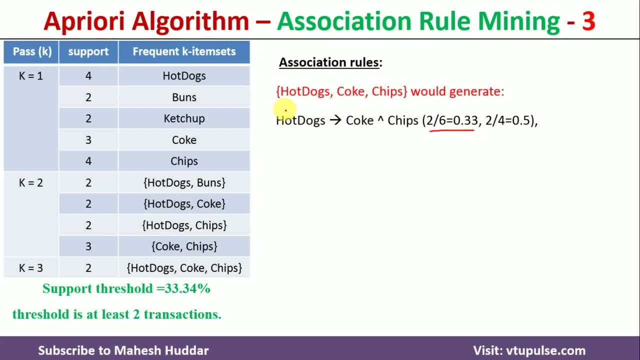 the number of times all three were purchased is two divided by the number of times hot dogs is purchased. that is the left hand side, which is equivalent to 0.5. again, it is less than the confidence coming back to the next one, that is, we will take coke this side, the remaining two on. 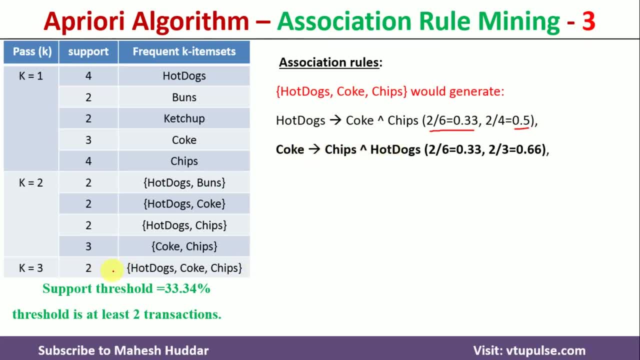 the right hand side, all three were purchased two times all the time. divided by six is the total number of transactions. the second one is: uh, all purchased two times and the number of times coke is purchased is three here, which is to 0.66. the meaning is it is the strong association rule. the next one is: we will take chips this side. 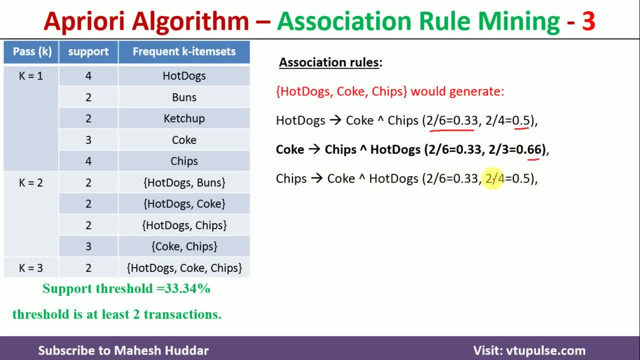 remaining all on the right hand side, and then we will calculate the support and confidence. so these three are over now. next, what we do is we will put two on the left hand side, one on the right hand side here, so hot dogs and coke on the left side. the remaining is chips here. so we 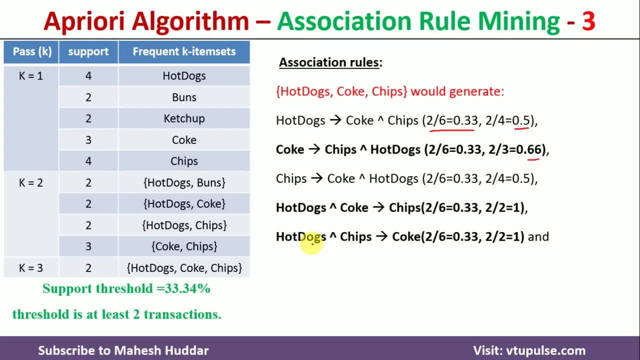 calculate the support and confidence. similarly, we will do it for the second possibility, that is, hot dogs, chips, right side coke. the next one is coke chips and hot dogs. so once we do this particular thing, we will get again four strong rules in this case. so this is the first strong rule. second one: 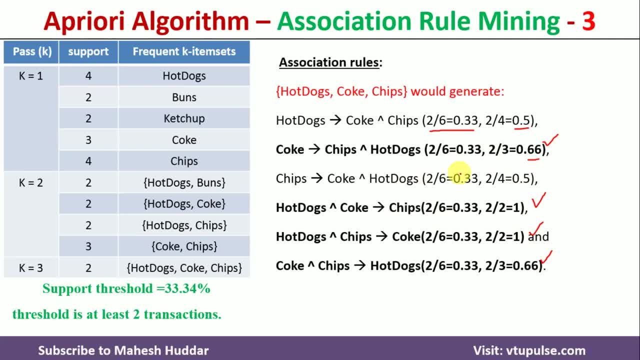 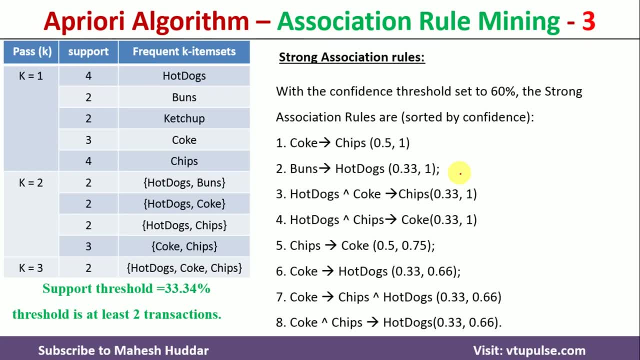 third one and then fourth one. finally, what we do is we will list out this particular strong rules based on the highest confidence here. so the first strong rule in this case is coke chips, because it is hundred percent confidence we got here. second one is buns, hot dogs- again it is hundred percent. 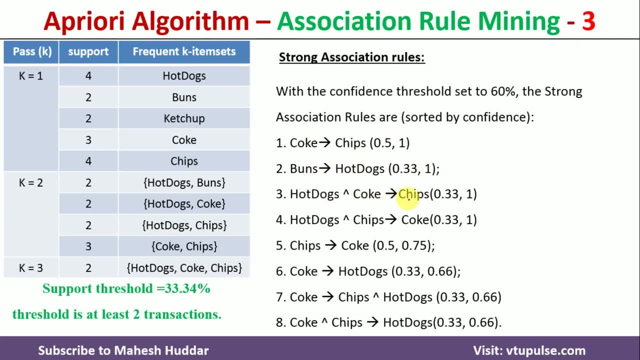 confidence, hot dogs and coke chips. this is the third one. similarly, we have listed all this particular strong rules because we have already calculated them in the previous cases here. so in this case i have discussed how can we apply the aprior algorithm to the given data set to find 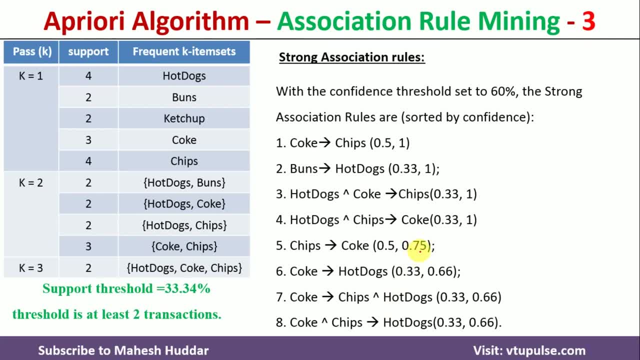 out the frequent item sets as well as the strong association rules. i hope the concept is clear. if you like the video, do like and share with your friends. press the subscribe button for more videos. press the bell icon for regular updates. thank you for watching.